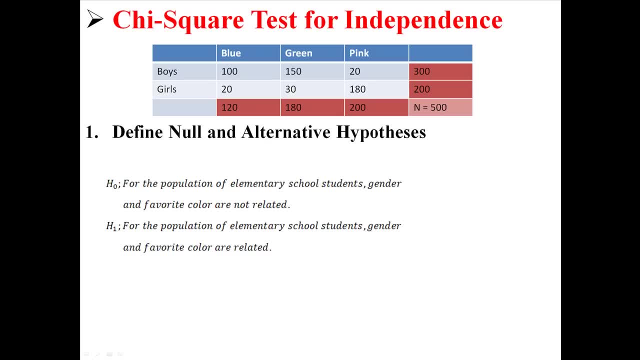 the population of elementary school students, gender and favorite color are not related. Our alternative hypothesis is that for the population of elementary school students, gender and favorite color are related. Now alpha, like I said, is always .04.. So alpha is .05.. Now, calculating degrees of freedom, we're going. 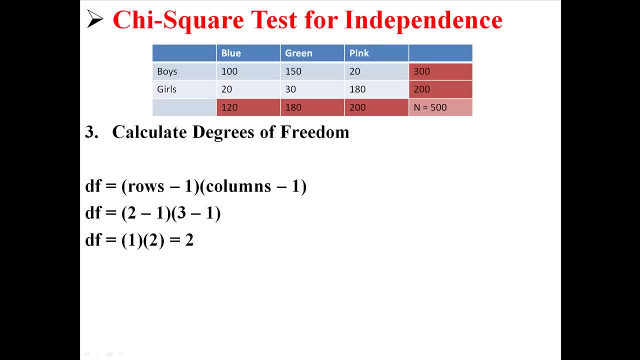 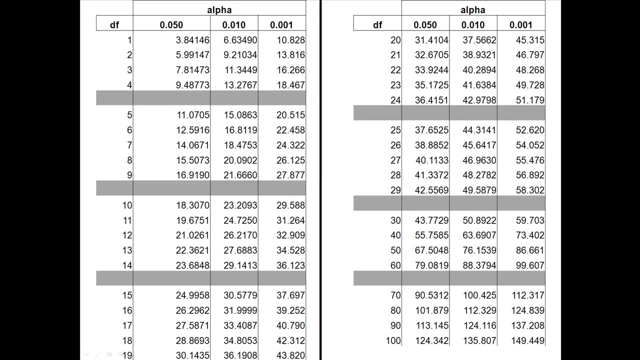 to take Rows minus one times columns minus one. Now we have two rows and three columns, So it's three minus one times two minus one, or one times two, which is two. This analysis will use two degrees of freedom And that's how we'll find our decision rule. We're going. 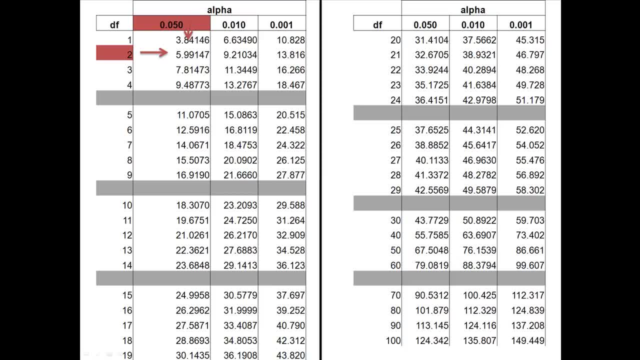 to go to our chi-square table and using alpha .05 and two degrees of freedom, we find a critical value of two degrees of freedom. So we find two degrees of freedom And that's value of 5.99147.. So our decision rule is if the calculated chi-square is greater than 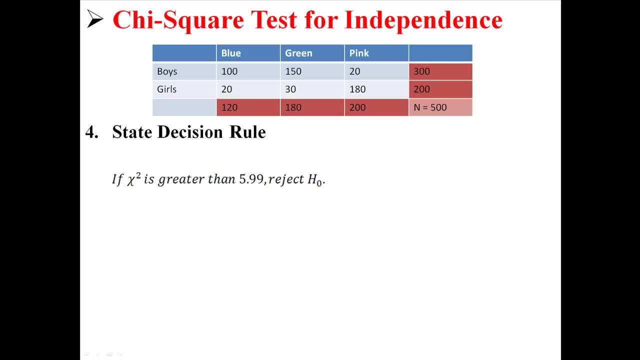 5.99,. we are going to end up rejecting the null hypothesis. So let's calculate our chi-square now. Now we're going to use the same equation to calculate chi-square, except now it's going to be a little bit more complicated to find the expected frequencies, And this is how. 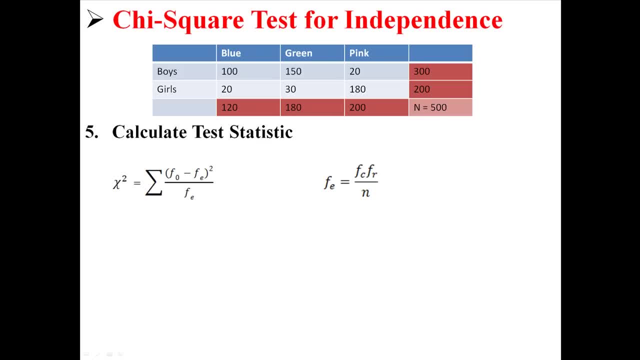 we're going to do it. We're going to multiply the frequencies for the columns times, the frequency for the rows and then divide by the total number of subjects to get the expected frequency for each cell. So, for example, let's say we wanted to find how many boys are expected. 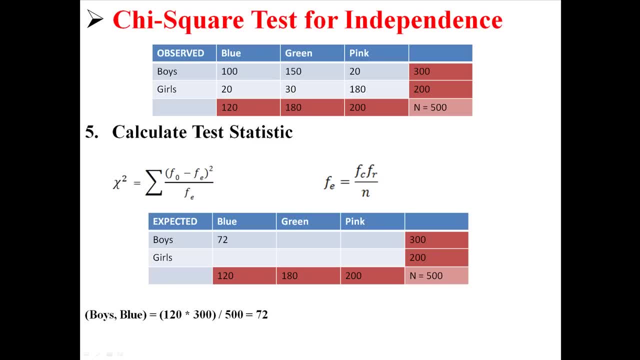 to have chosen blue as their favorite color. We take the column total for blue, which is 120, and multiply it by the row total for boys, which is 300, and then we divide by the total number of subjects, which is 72. And we find out that in this sample we would have expected 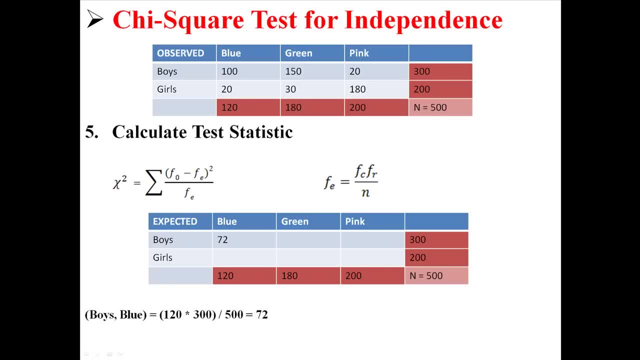 72 boys to choose blue as their favorite color, And then we can continue that to get the expected values for all 6 cells. So now I'm just going to move that up and we have the observed values and then, next to them in parentheses, we have the expected values. And now we're going to